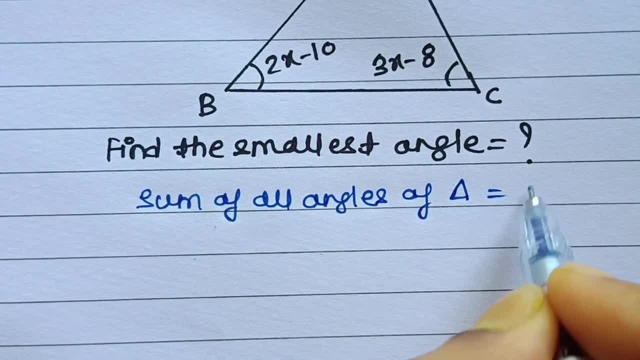 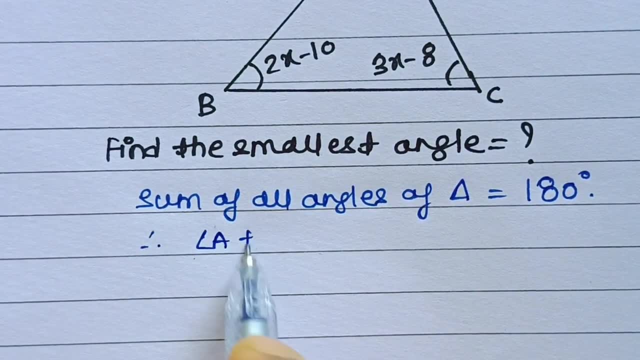 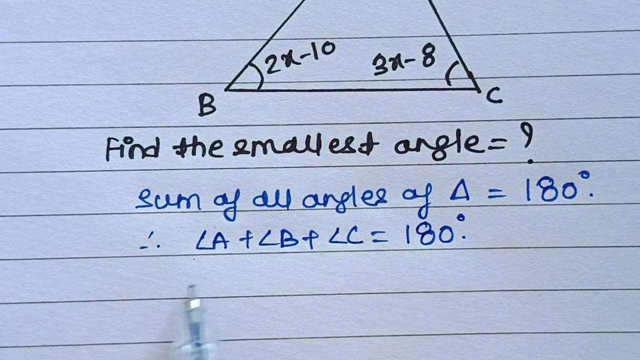 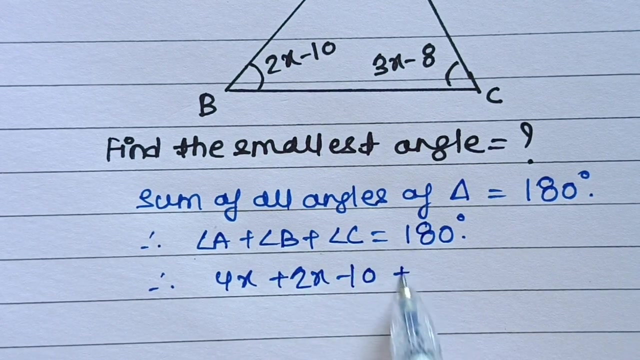 to solve by your own. Now let's see the solution, As we all know that all the angles of a triangle equals to 180 degree. Therefore, angle A plus angle B plus angle C equals to 180 degree. Now we put the value of individual angles: 4x plus 2x minus 10 plus 3x minus 8 equals to 180.. 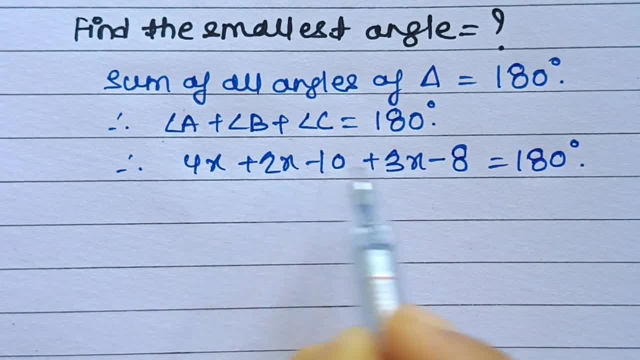 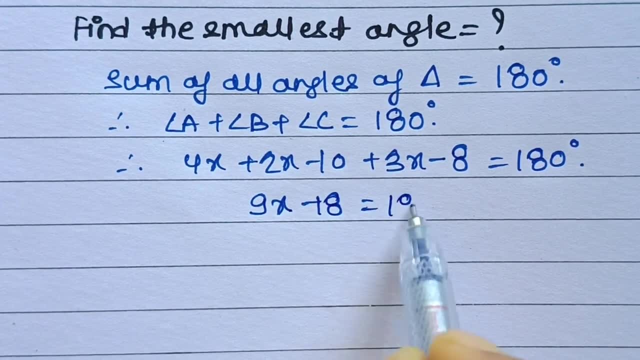 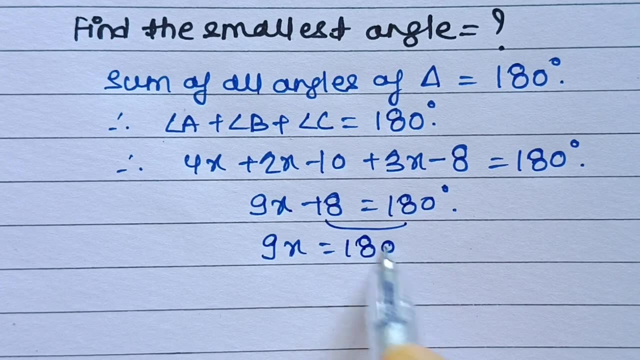 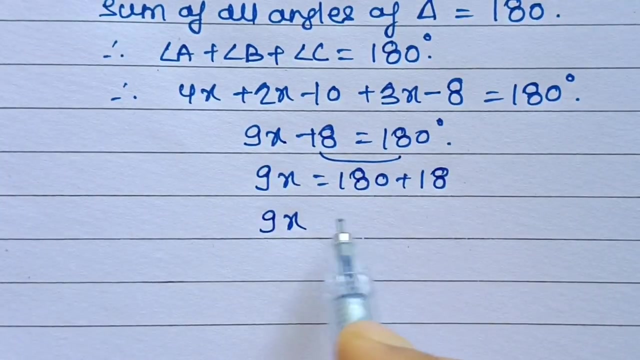 Now we add the coefficient that contain x, that is 4x plus 2x plus 3x, it's come 9x minus 18, equals to 180 degree. Now we take this minus 18 to the next side of the equation and it's come 180 plus 18.. Now the equations become: 9x equals to 198. 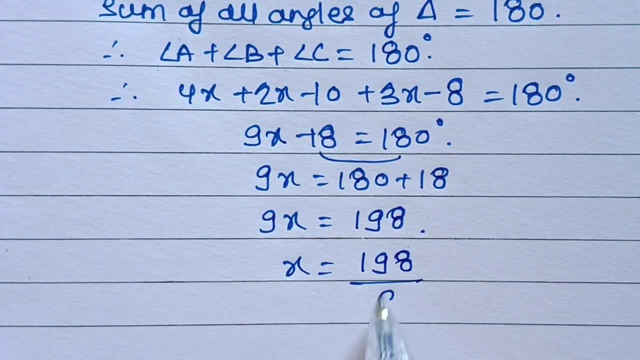 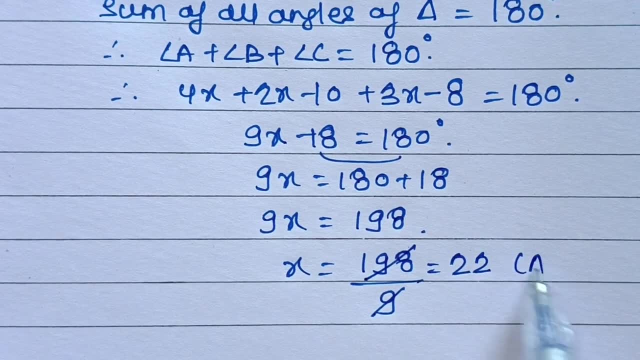 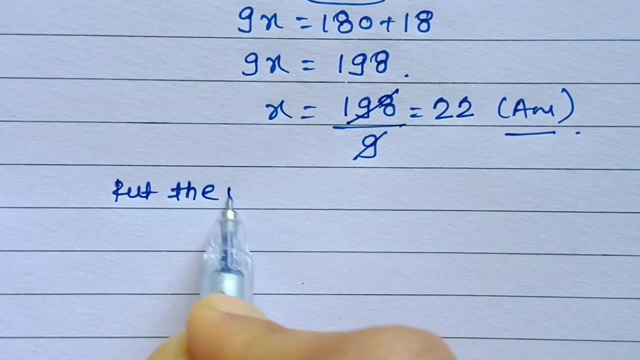 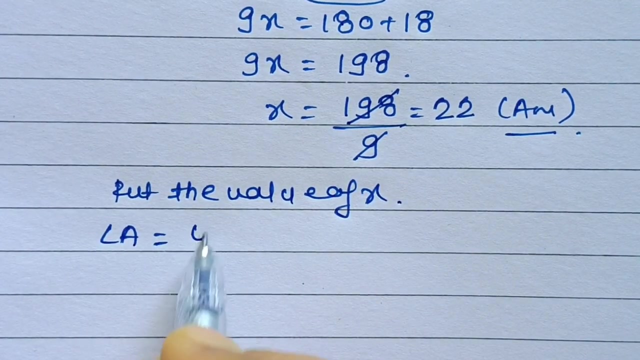 So the value of x come 198 divided by 9 equals to 22 degree. Now we put the values of x to individual angles in order to find who is the smallest angle among them. Now the value of x into angle a equals to 4x. equals to 4 x 22 degrees equals to 88 degrees. 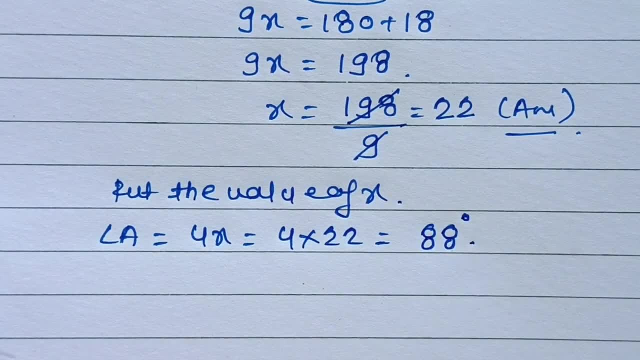 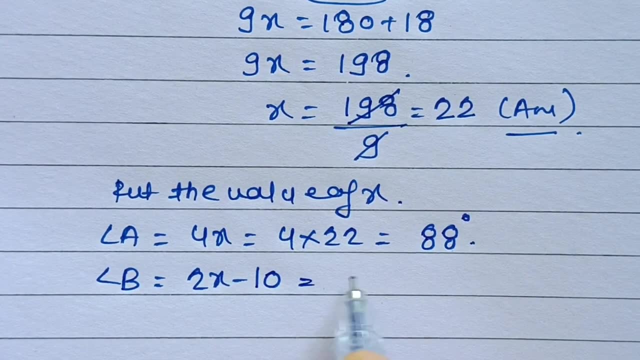 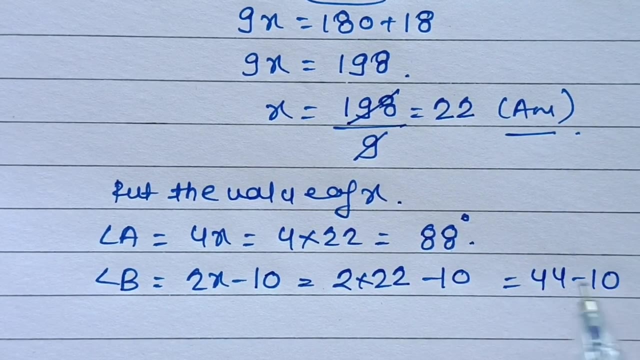 Angle B equals to 2x minus 10 because angle A equals to 3 so when we take a 4x result, we consider the value of 2x equals to eran angle �. 10 equals to 2 multiplied by 22 minus 10 equals to 44 minus 10 so the value of angle B comes 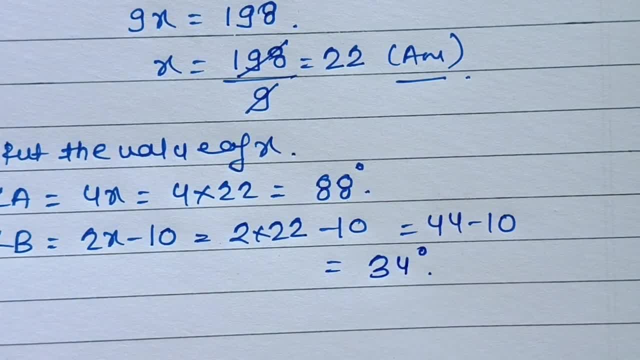 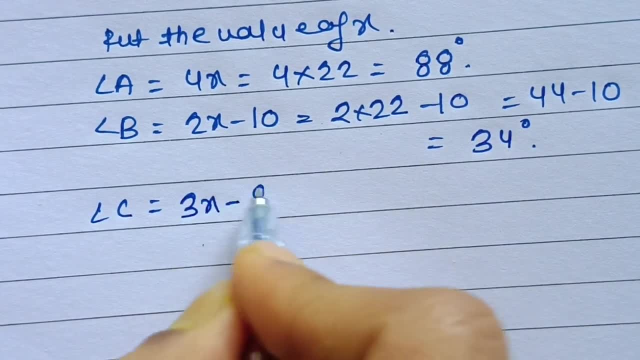 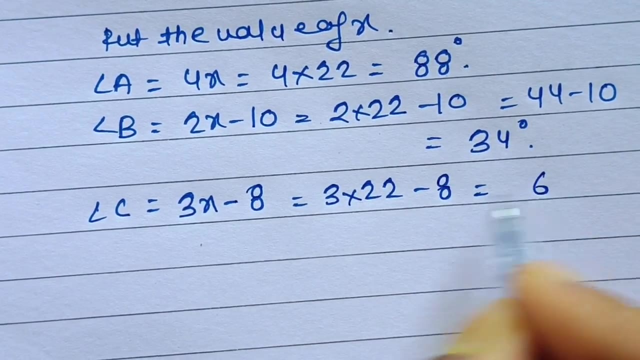 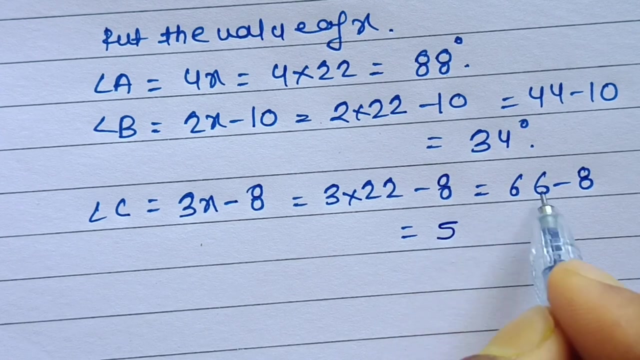 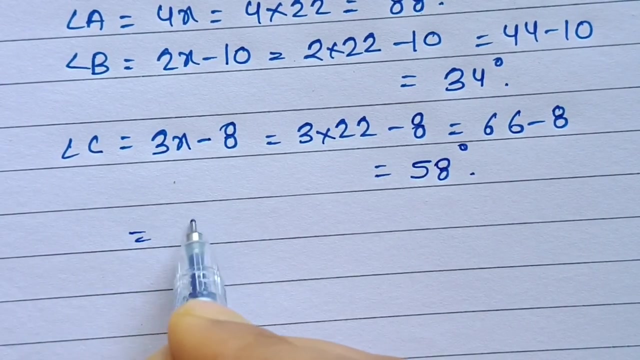 34 degree and the last angle C. angle C equals to 3x minus 8, so it's come 3. multiplied by 22 minus 8, it's come 66 minus 8. so after subtraction it's come 58 degree. so the angle: